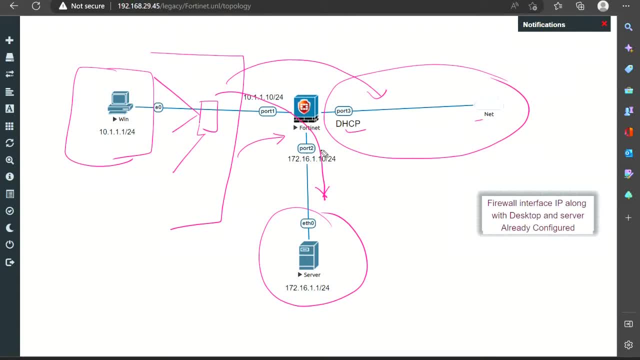 here and without this one. let me show you first that how, without configgram firewall, are they able to ping these ip addresses or not? and after configuring the policy that, are they able to ping or not. so let me clear this one and let's switch to the gui of the 48 firewall. so this is my gui. it has. 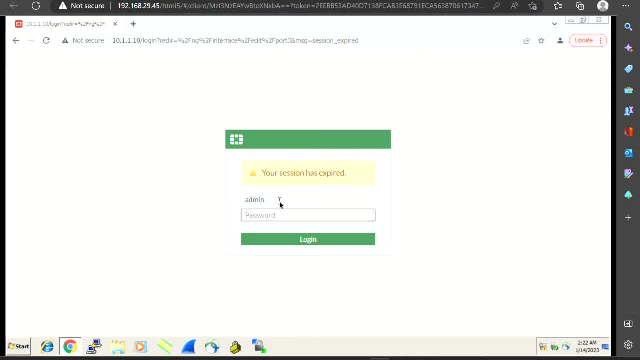 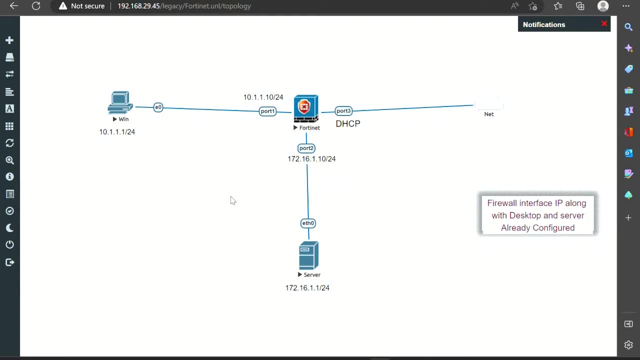 timed out, so let me log in it. and, just for the sake of convenient, i want to tell you that i have configured the ip addresses on the 48 firewall and i have configured the ip addresses on the 48 firewall. all these interfaces of the ip address, along with the 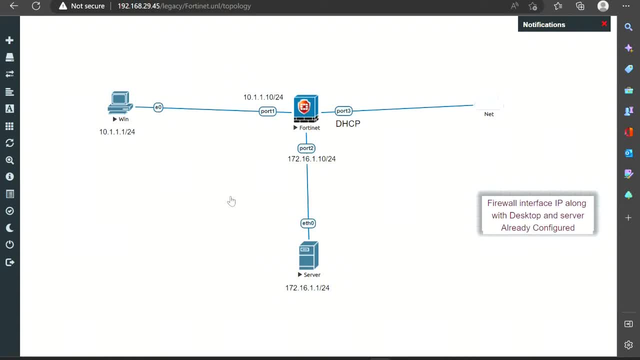 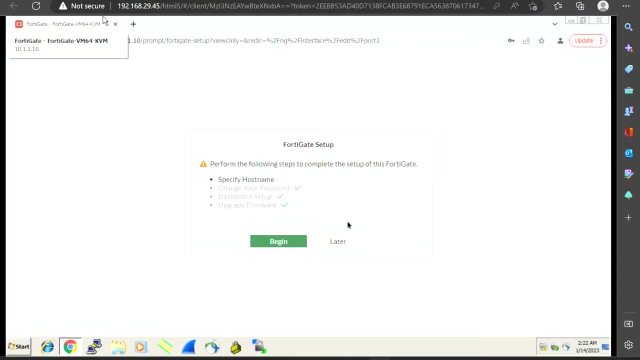 this machine and this server here right, and how to configure the ip addresses on the network interfaces of the 48. you can watch my previous video. i have another session for that one and as of now we are just focusing on the firewall policies, so i'm not going to change any host name. 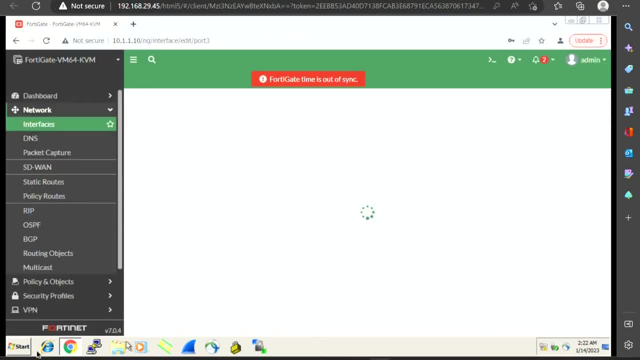 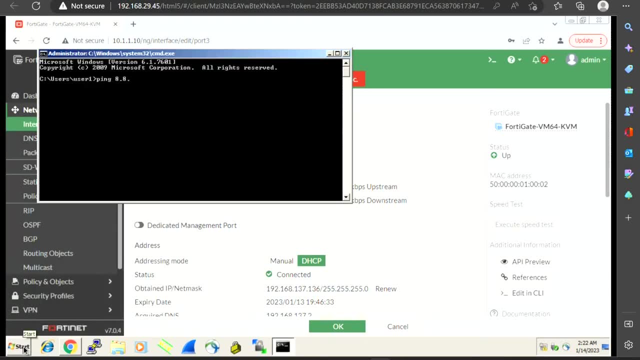 or something. i will just simply go to the firewall policies. so, as of now, let me show you that. are we able to ping the internet currently or not? so let's go to the firewall policies and let me show you so. internet ip address: 8.8.8. as of now, i'm not able to ping it here. and let me open. 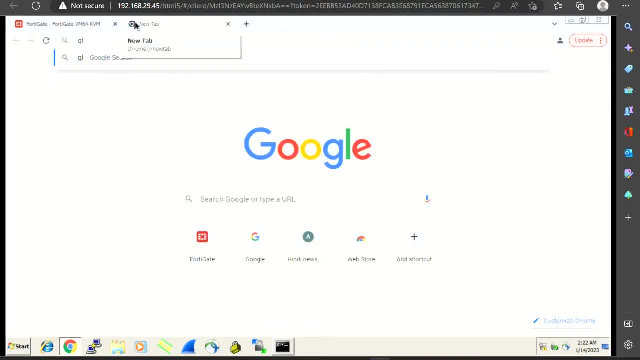 googlecom. are we able to do it or not? don't get confused with the background page. i'm just opening the googlecom and as of now, it should not be allowed because we don't have any firewall policy to allow it. it's taking some time, seems like that one that it is will not be allowed. 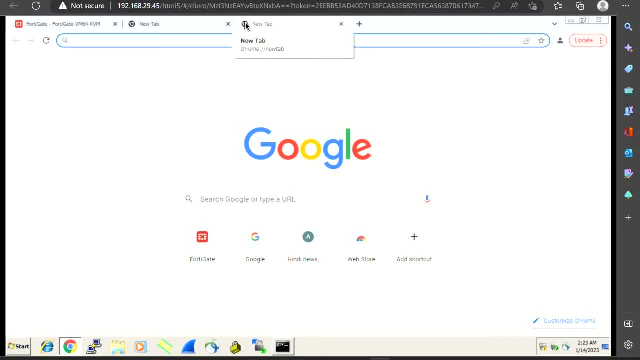 right. so that's why it is taking time. let me take another website like cnn or something. try to search anything. anyhow it's taking time. but let me tell you that it is not going to open because we don't have any rule allowed through the firewall and by default in the firewall we are having the implicit deny. 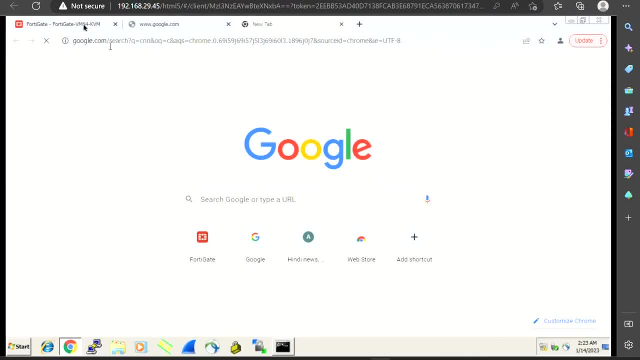 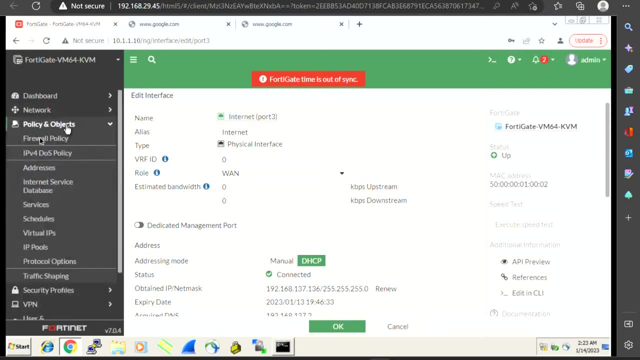 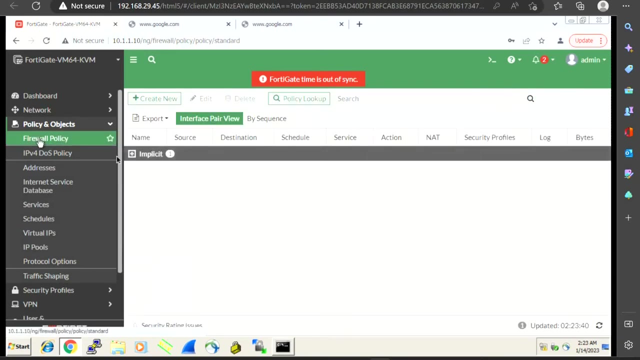 policy and it does not allow anything to pass through the firewall. so let me show you that first, for that one, we have to go to the policy and objects let, and there we are having the firewall policies. all right, so as we open the firewall policy, we see that we have only one default policy, that is implicit. deny that traffic. 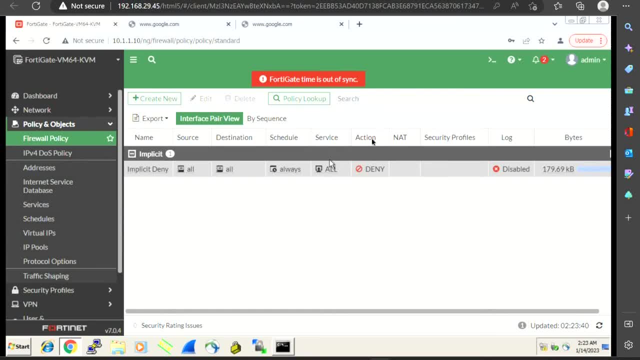 from any source, any destination, any service. always, action is deny right. we don't want to pass any of the traffic through our firewall without our policy, so let me show you that permission. so for that one, we are going to configure one firewall policy and i am going to 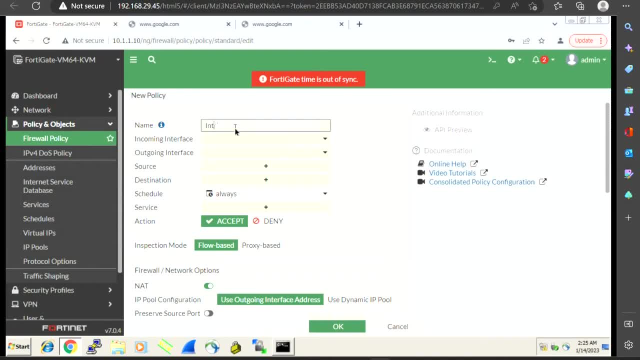 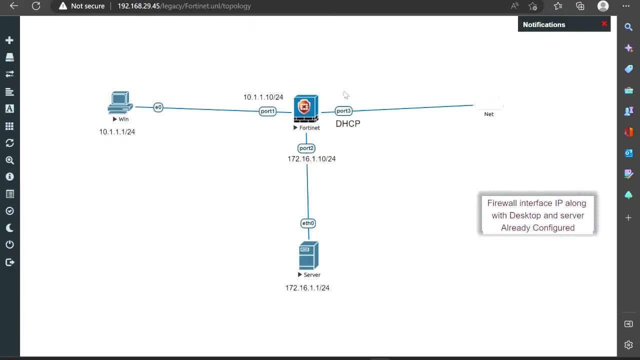 create. put on click on the create new name, first one. i am going to do it for the internet incoming interface. i want to put it as a port one. outgoing interface is for the internet. it is port three. let me show you once again: incoming interface is port one here. outgoing interface. 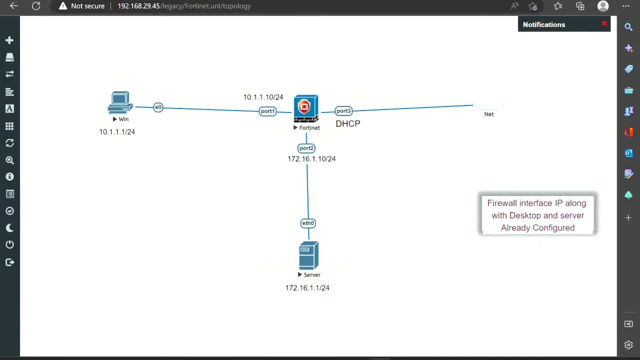 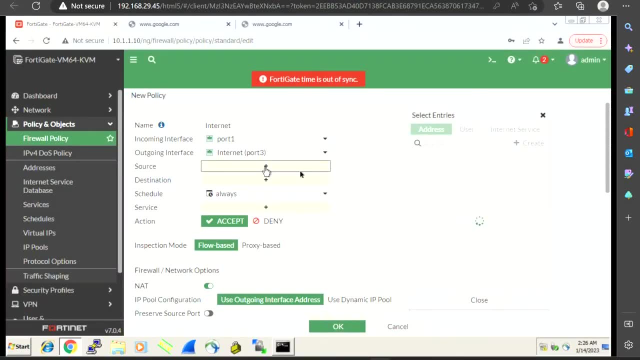 is port three here. that is basically a dhcp ip address. so all right, and the source address. we can create a subnet for that one. i have created a address group 10.1.1.0. let me show you how to do it. you can just simply. there's two ways to. 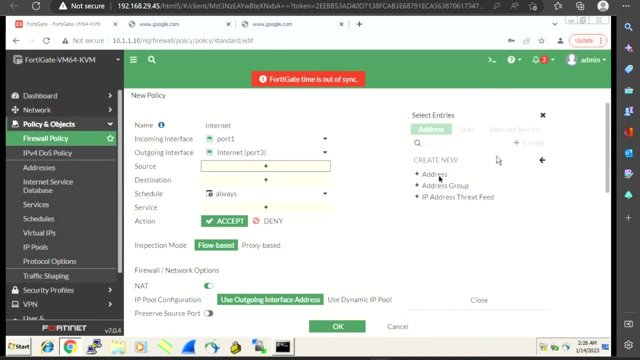 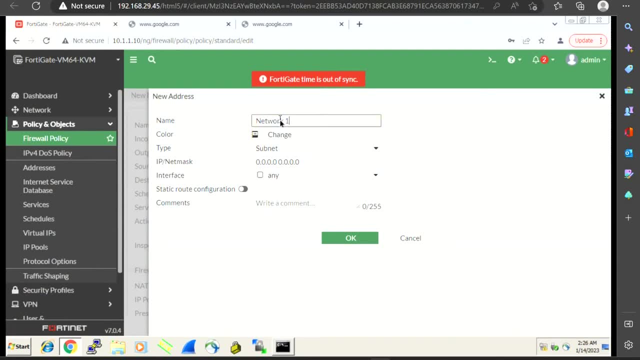 create it either. we can do it from here directly: click create address and you can give any of the name, like network 172.16.1.0. so this is the name of the address group, and we can create a subnet for network i am creating, or let me put it like network underscore and underscore net. this is 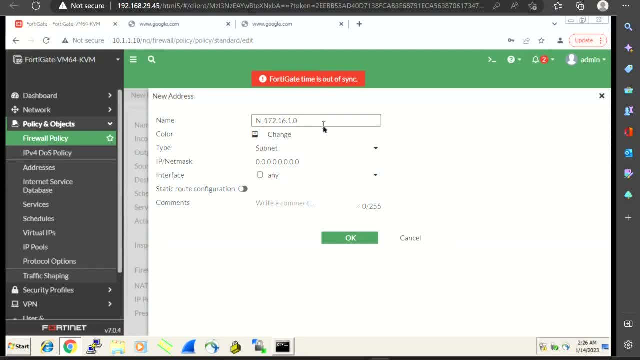 actually the for the sake of convenience that whenever next time anyone viewing this object, they can just let us know that this is n standing for network. that is not any specific ip address. right type subnet. i want to choose it here, i don't want to. we can choose it here. ip range as well. 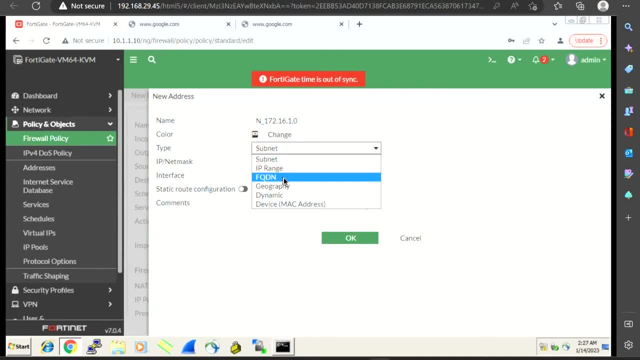 fqdn. fqdn stands for the fully qualified domain name, so we can directly put it any domain name here, rather than giving the ip address. so these are the options we are having. so as of now, i am going to use subnet here and the subnet we are using 172.16.1.0, and subnet mask. 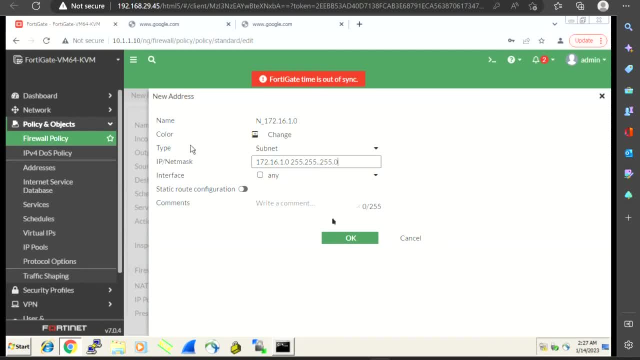 255.255.255.0. that's it and just hit ok comments. if you want like something, you are on the any change window and you want to mention any change number here and that this is the change number which you are doing that one. so for that sake of comment section is there, you can use it. 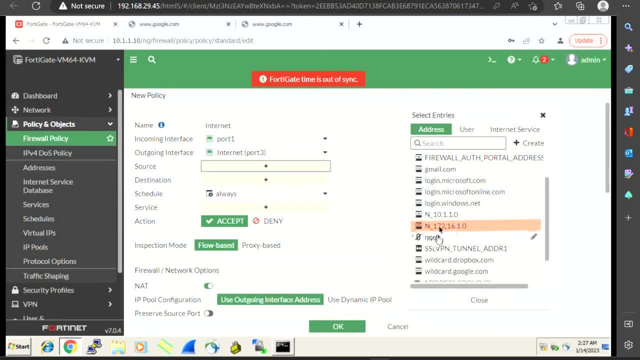 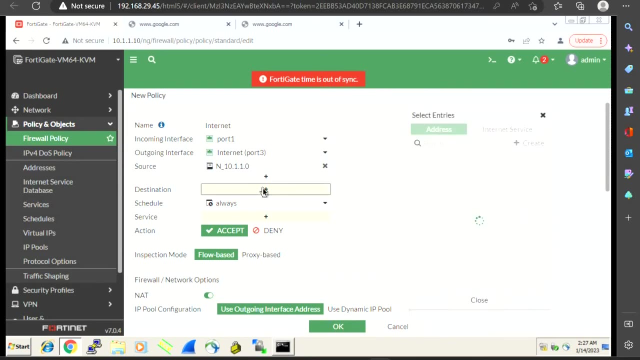 now it is created. i'm not going to use this one. this was just to show you, because for this policy we don't need it here. i'm going to use the object, this one, 10.1.1.0, because my computer is under this network destination. i want to put it any. i don't want to block any of the traffic here, so 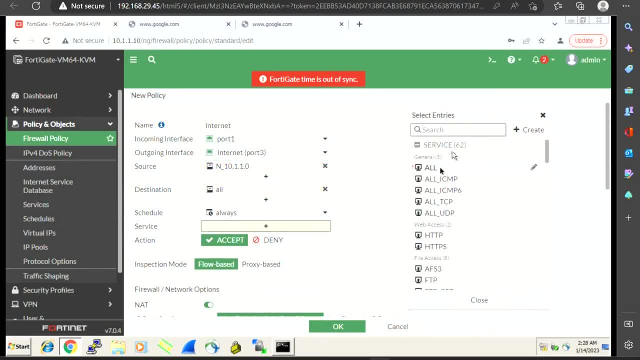 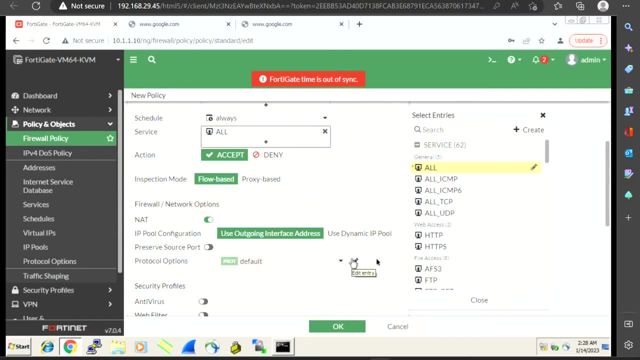 that i can drag and drop here all the services i want to allow. i don't want to allow any specific, i want to allow the users to use all the services. next thing is very important, which is nat part here. so here, for the sake of convenience of the internet, i'm using nat here and use outgoing 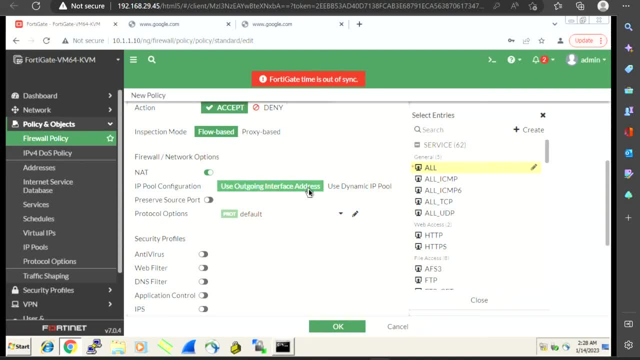 interface address. so this is a part of nat that if you are very good in the nat, then you can understand it. if you don't want to, if you don't know the nat, then not to worry, just enable it. this is just for my lab set up, so i'm going to use this one, 10.1.1.0 and subnet mask. 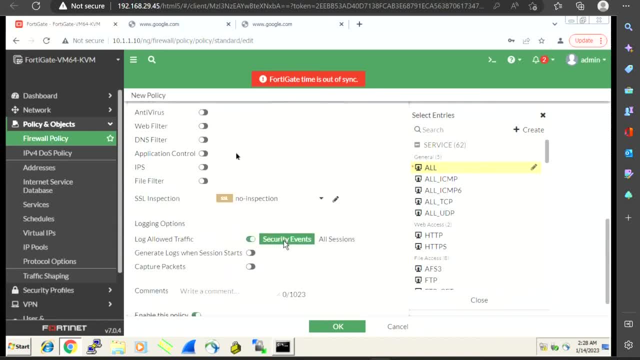 this is basically so that i can use the internet, and just, these are the security profiles. i will explain it later on that. what are these? basically, if you want to use it under this policy, we can enable and use it. we want to enable or disable this policy. so by default, if we hit, ok this policy. 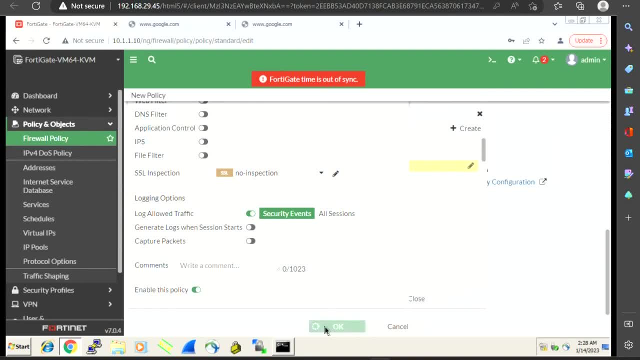 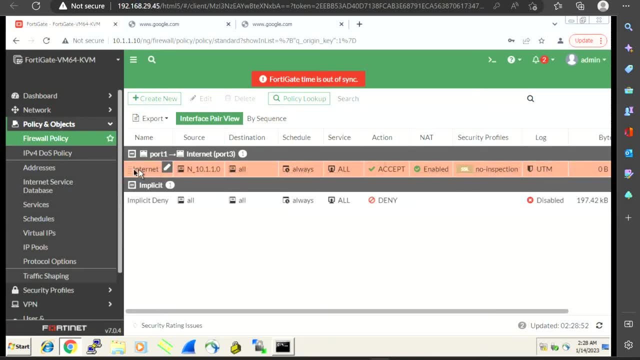 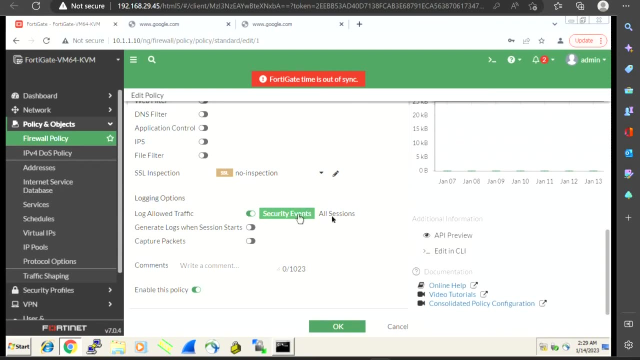 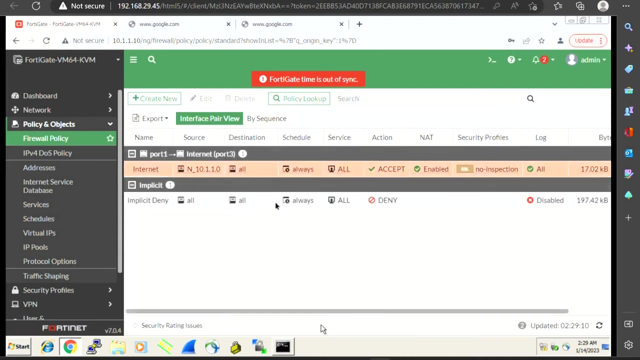 will be enabled and we want that one. we just hit ok, so this will. but one thing i forgot: i want to log this traffic as well. so this is currently under utm, that only security events will be logged, but i want to log all the sessions, not only security events. so that's all set. and that's one more thing to note whenever 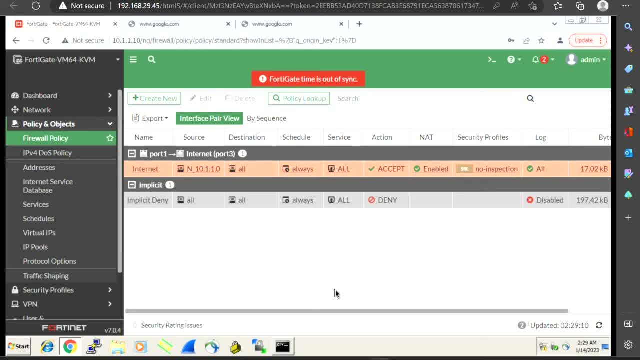 we just hit ok, we don't have to do any save or commit changes, something like that one, or push anything on the firewalls. once we hit ok, everything is applicable on the firewall. so this is very important whenever we're doing something like that, we don't have to do any save or commit changes. 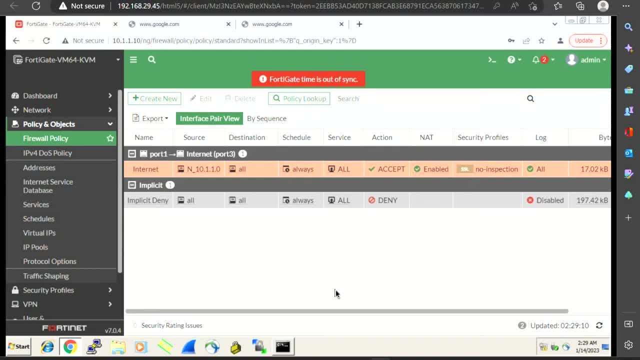 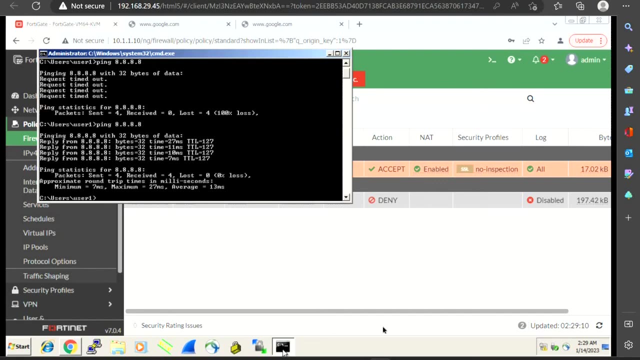 we should be very careful, uh doing this configuration, because they are, they will be impacting your production environment. immediate effect, right? so let me just show us that. are we able to ping it now 8.8? yes, we are able to hit 8.8. it means that we are having access to the internet. 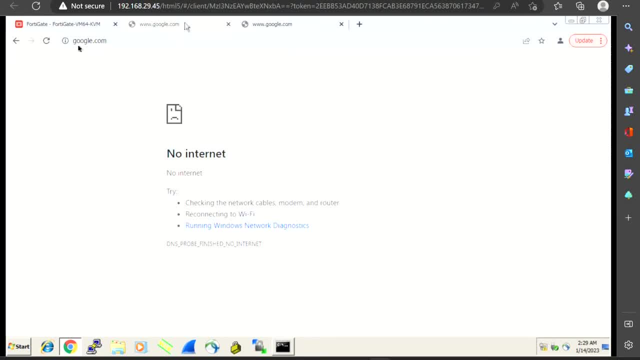 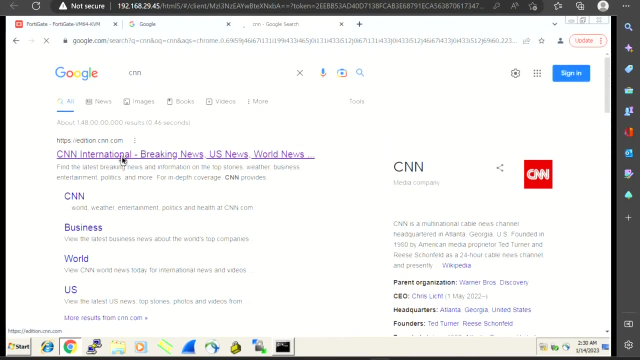 so let me just check it that whether previous one, so previous googlecom, was not successful, oh, now it's successful. just after our firewall policy and now it we can open any of the website perfectly. it is opening. there's no issues in that one. yeah, one more thing that it will give, i think. 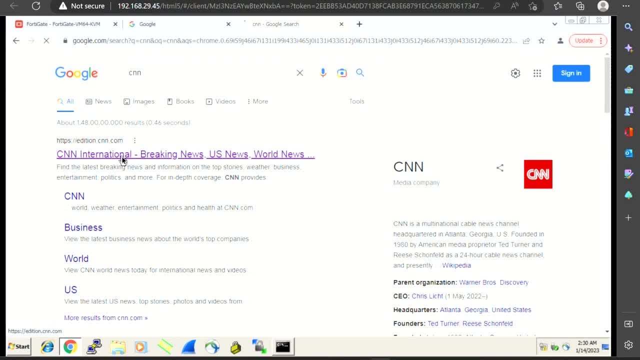 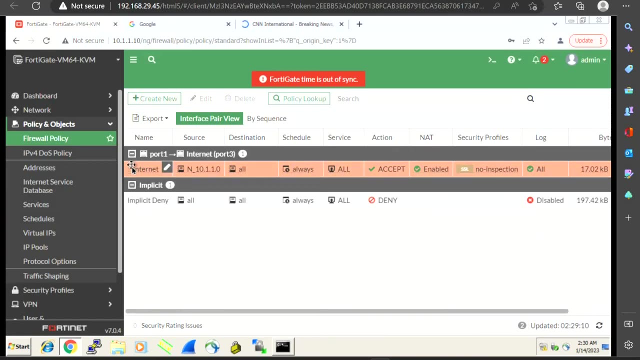 security error, most probably because we have enabled the ssl inspection. so don't worry about these things. we will cover it later on in the later on videos. so it is giving a security error because we are, we have enabled the ssl inspection and we have enabled the ssl inspection and we have. 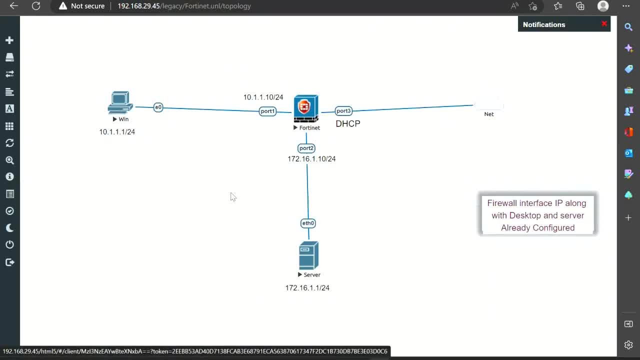 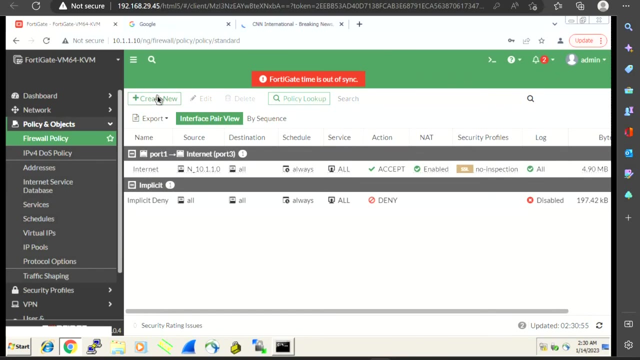 enabled the ssl inspection here. that's it. i think from this one i want to create one more policy for the dmz server. as of now. let me just do it that as well. let me create one more policy, create new. so this one is for the dmz connectivity. 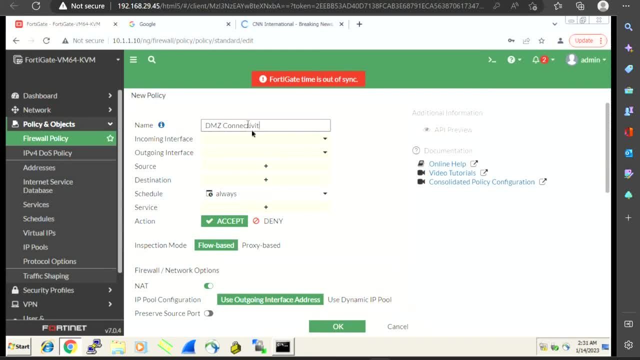 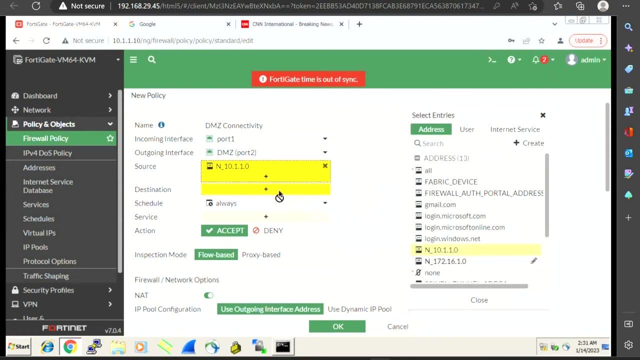 incoming interfaces. port one- that's fine- outgoing interface. this one is, i think, port 2 dmz. let me cross verify. yeah, this is the port 2 and the source. i want 10.1.1.0. that is my source here, this network, and 172, this one. 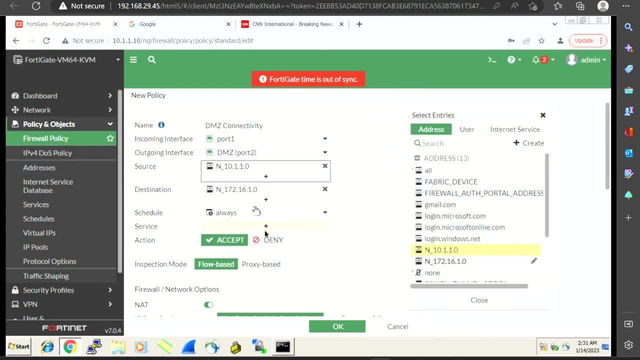 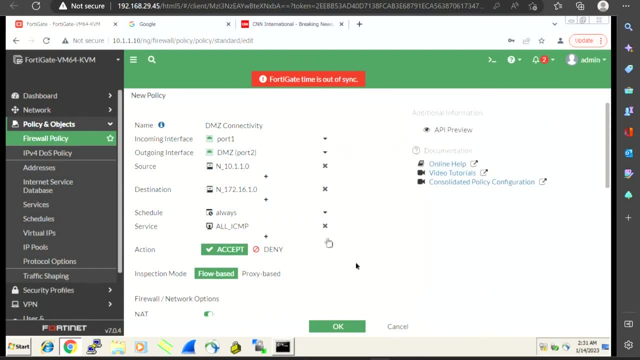 perfect and services any, all the services i want to allow, or let me just allow only icmp remaining. nothing is allowed. all right action is accept. i don't want to enable nat this time because that will be accessible. no inspection. allow all the traffic and log all the sessions. enable this policy hit ok. 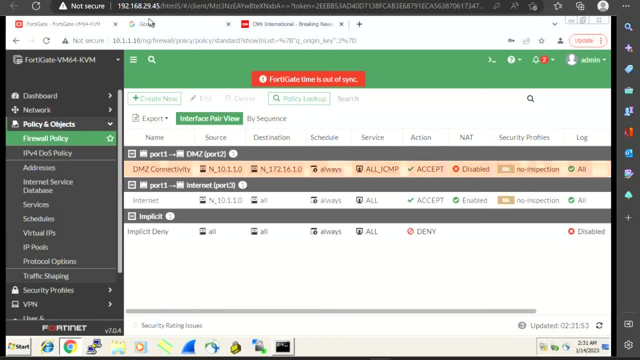 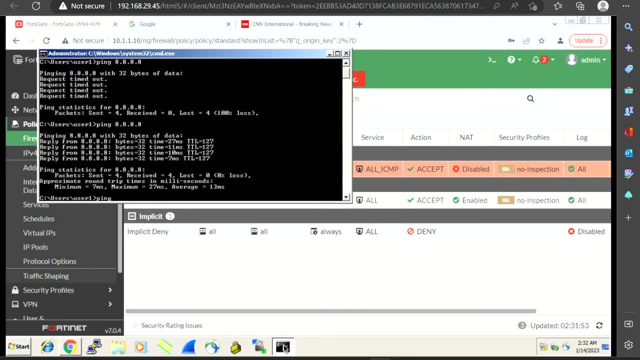 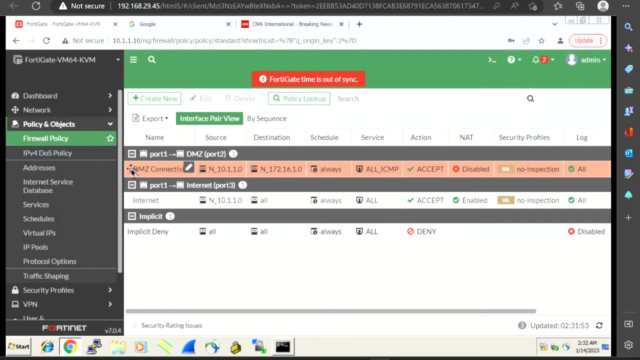 we have this policy. now let me just ping our machine and that should be pinging. let me just check it. 172.6, 16.1.1, i think it was, and now it is there. it's pinging without any interruption. let's just disable this policy and then check it. are we able to do it or not? 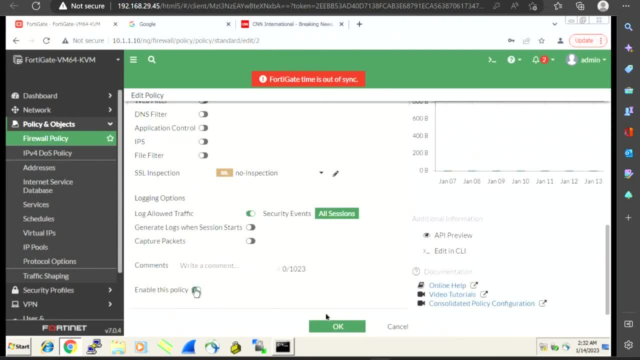 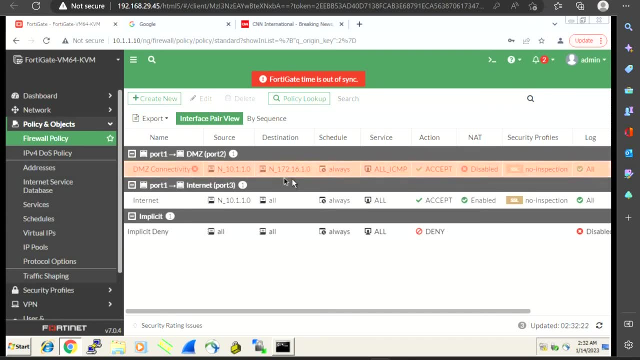 let's disable this policy hit ok, we have the policy. this is the benefit of like disabled feature. we are having the policy, but this is disabled means that this is not taking any effect. now let's try to ping it now that, are we able to do it or not? 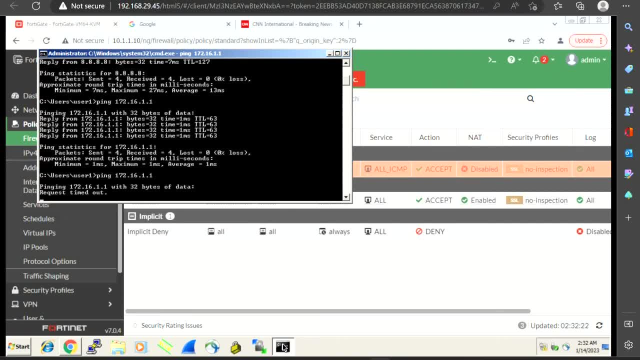 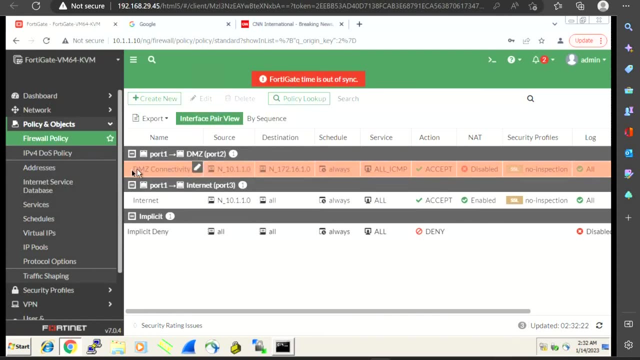 and here we go, it's working, our firewall is working very fine. it is denying the traffic and we are not able to reach our dmg server. so this is the basically no scope of firewall policies. one more thing let me just tell you, or show you, basically. so let me just enable. 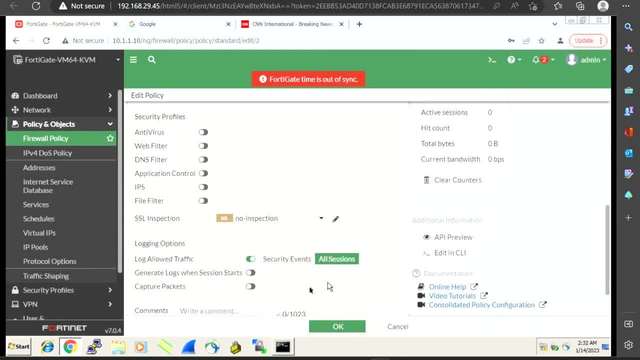 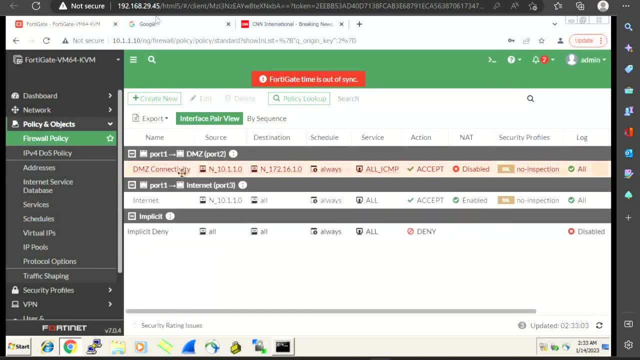 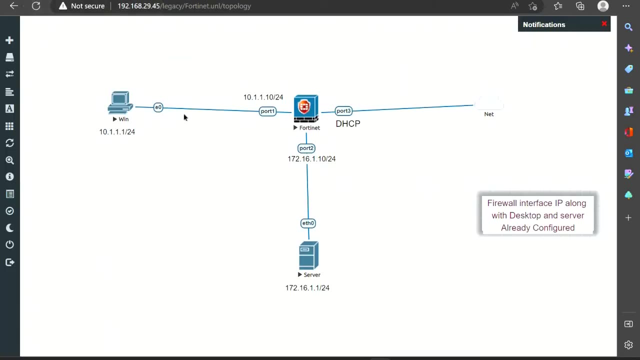 this policy and hit ok. so this is applicable now and now. let me show you this scope of these security policies, that how they are actually working. so now we are having a policies to allow it from here to internet. we are having the policy allowed. we have a policy to allow this traffic. 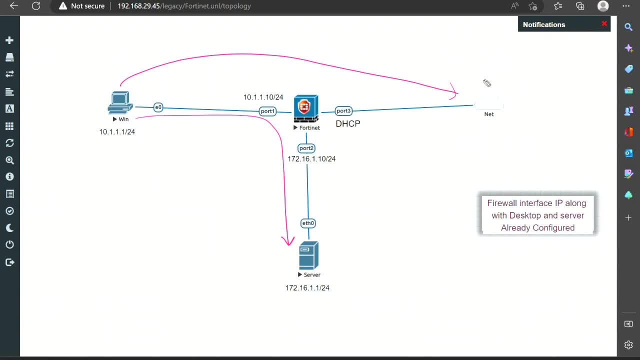 to here. so these two ping are working very fine. we are trying to ping 8.8.8, but we don't have any policies to go to internet for this dmg server, right? so what you guys say that if we try to initiate ping from here to 8.8, will it be working or not? 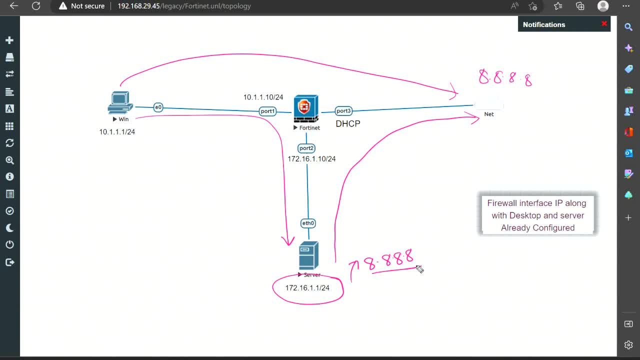 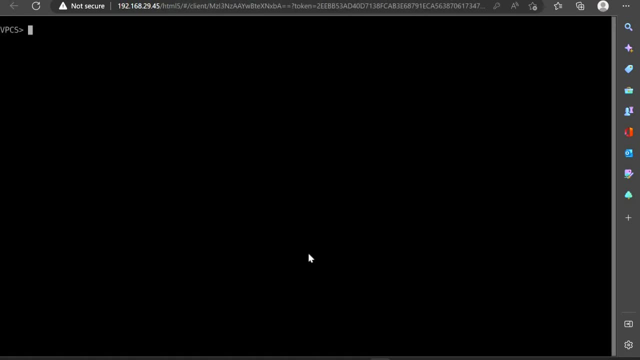 what you say. yeah, it will not be working right because we don't have any firewall policy allowed for that one. let's just do it. ok, let me open. this is basically virtual computer. i have taken it like as a server. let me try to ping it from 8.8.8. 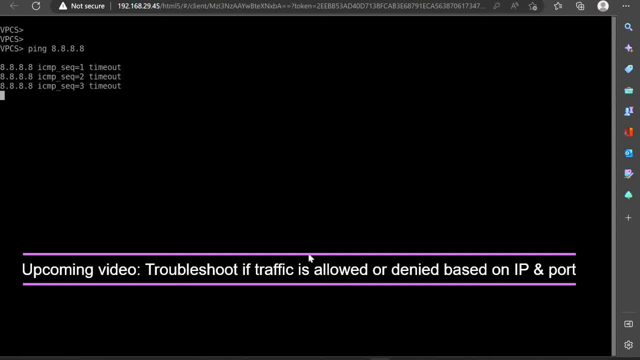 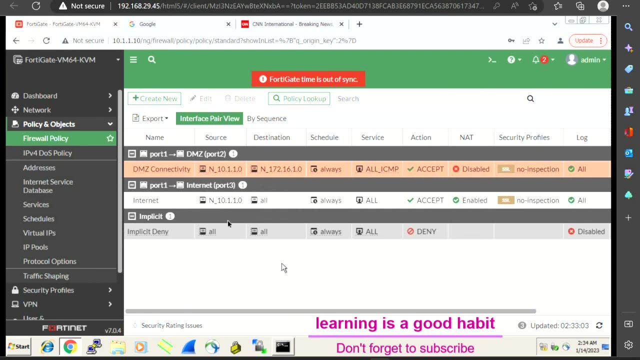 and it shows. it says that icmp is timed out. now it's your requirement, from your organization, that you want to allow this machine to reach to the internet as well. what will you do, right? so what you're going to do? are you going to create a new rule? no, mate, you don't have.